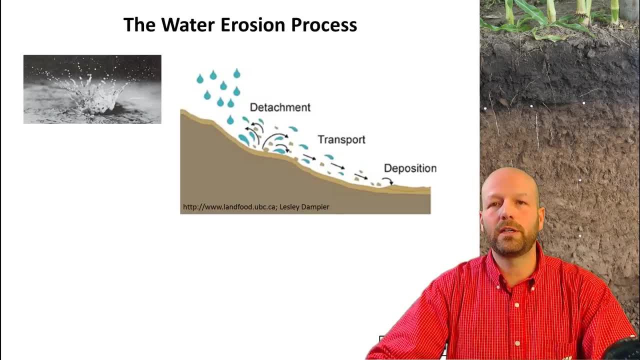 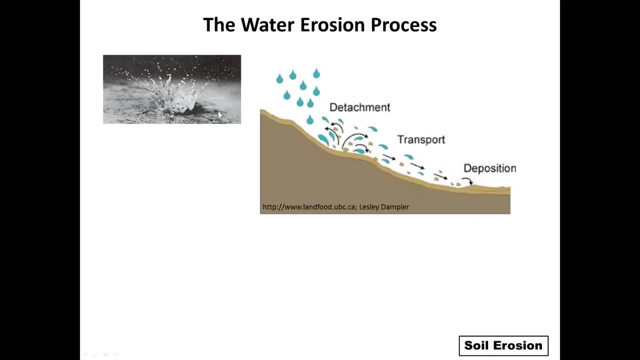 So let's talk about water erosion in a little bit more detail. So, looking at the water erosion process, it's actually a three-step process. So the first thing that happens is detachment, So that's caused by the impact of the raindrop. 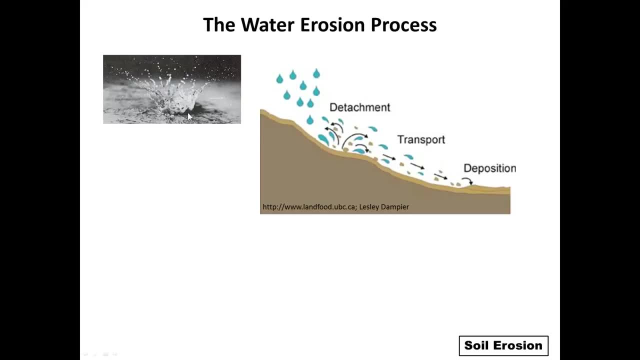 It hits the soil surface and it'll detach sand or silt particles or clay particles out of the soil. So if you recall on your basic soils, if you had a soil that has good aggregate stability, those soils will actually resist this detachment force a lot more than weaker soils. 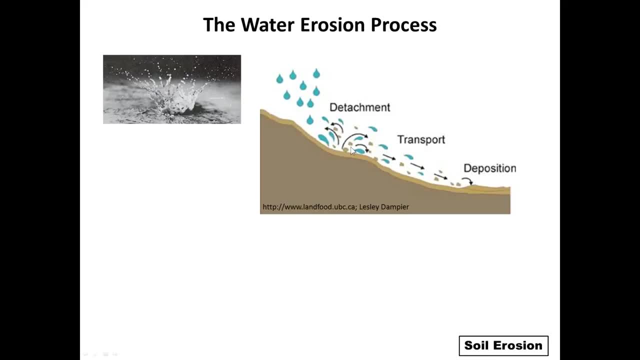 So once that soil particle is detached, that particle can be transported. It will be transported and will move from the field and it will get deposited. So the other two steps of water erosion will be the transport and then the deposition of that particle. That deposition could be in the field, in the same field. 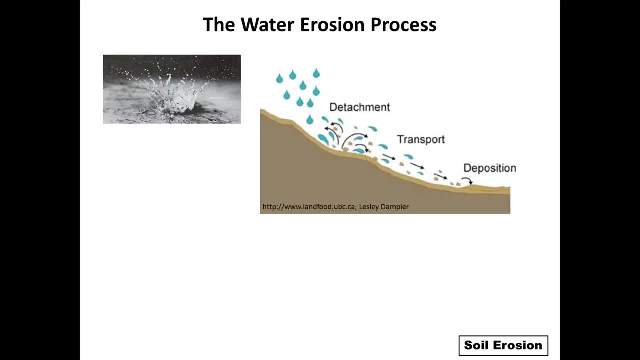 It could be in a waterway or it could be deposited in a stream or lake. So in my opinion, once that particle gets detached, we are already losing the battle with soil erosion. So you might have heard of the USLE, or Universal Soil Loss Equation. 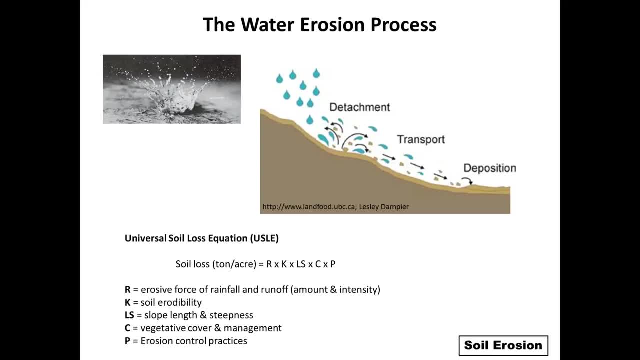 I think it's a great way to look at things that we can do and how we can manage erosion by water, And you can see the formula here in the bottom, where we have the soil loss in tons per acre equal to these different factors: R, K, L, S, C and P. 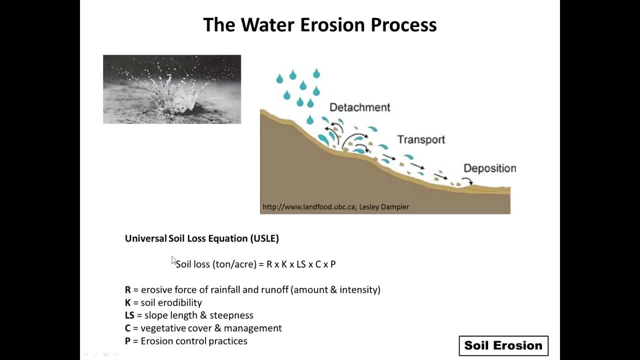 R being the erosive force of the rainfall water and the runoff. So the amount and intensity, K is the erodibility factor, also how erodible your soil might be. L S is the slope length and steepness. 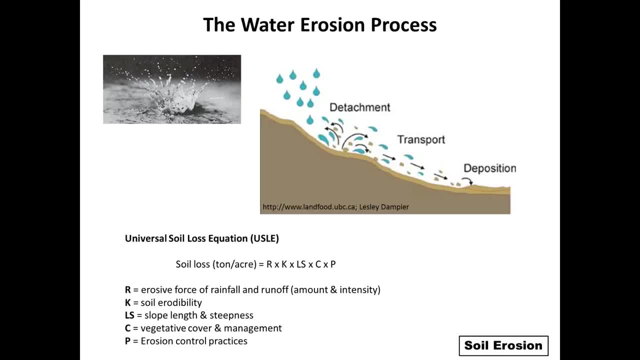 C would be your cover and management, So residue on the surface, what type of crops you're growing. And then P would be your control practices, And we'll touch on some of these as we go along. The USLEs have been revised right now and it's called the Revised Universal Soil Loss Equation 2.. 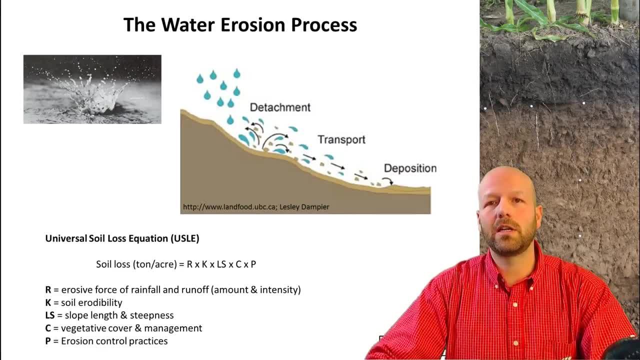 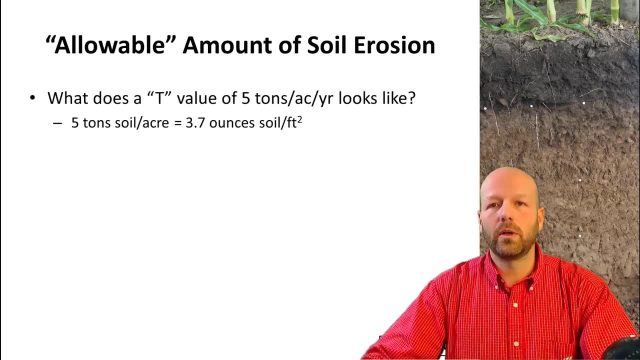 And it's a little bit more complicated than this, but I think this USLE concept helps us look at erosion and kind of think about how we can manage soils to reduce erosion. So in Wisconsin usually what we call the tolerable soil erosion or the soil erosion equation. 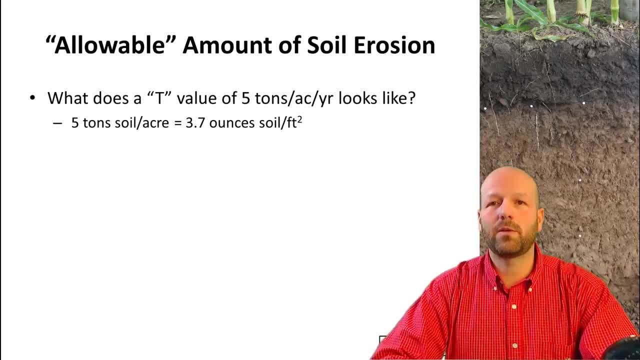 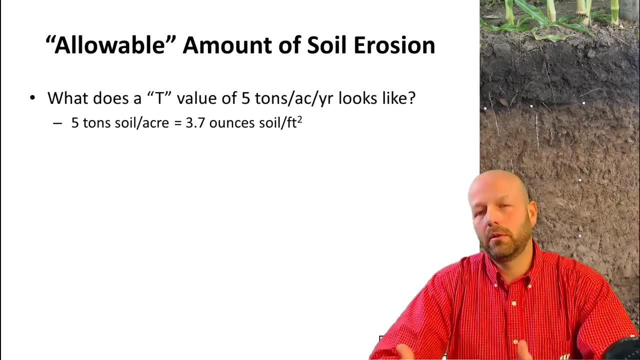 what I showed you: soil loss. it varies anywhere between 3 and 5 tons per acre per year. That's what we call tolerable or allowable. However, you know me, I have a hard time, even as a little scientist, wrapping my head around that value. 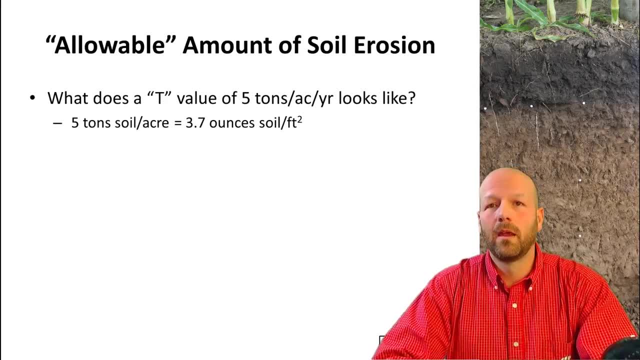 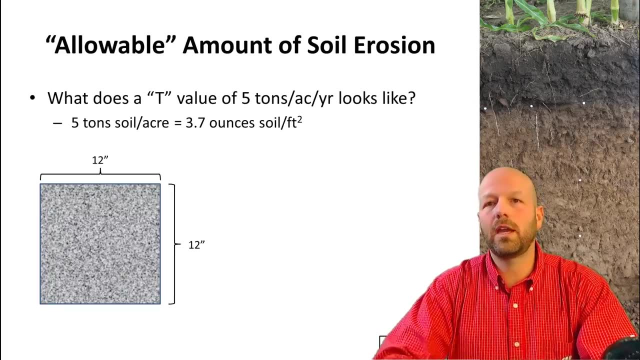 What does 5 tons of soil per acre look like? So if you were to calculate that on a square footage basis, that's about 3.7 ounces of soil. So if you were to take a floor tile, a 12 by 12 floor tile- 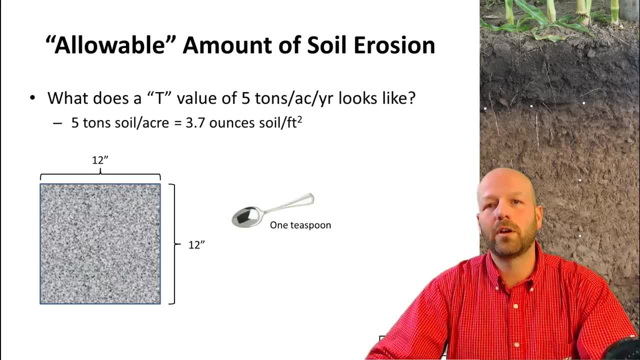 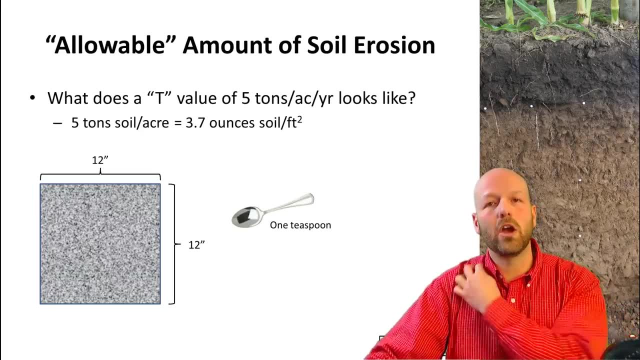 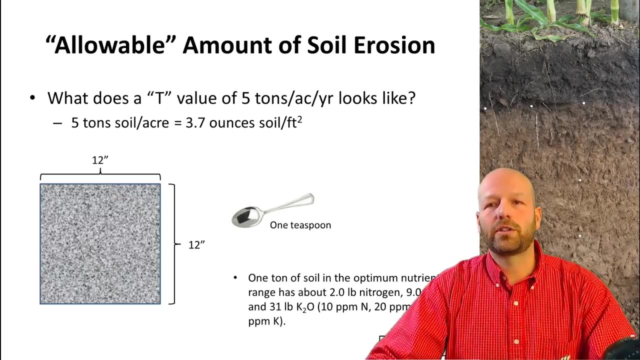 all you would need is about a teaspoon of soil, And that would be equivalent to 5 tons of soil per acre. So, as you can see, it doesn't take a whole lot to lose beyond those losses that we call tolerable. Now, taking it another step further, 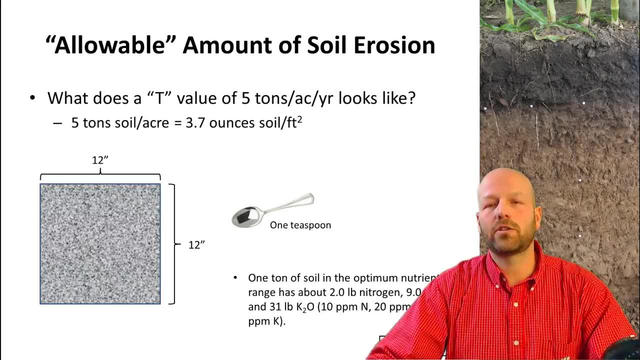 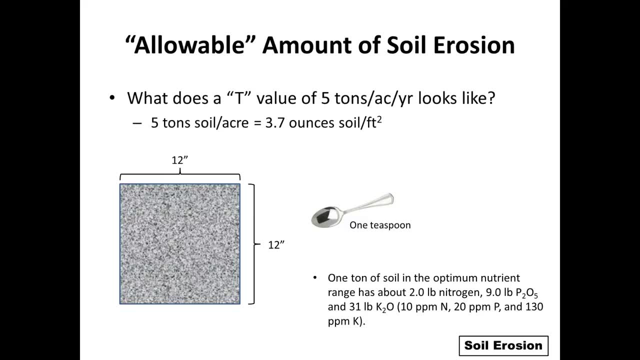 we can see that the value of the fertilizer, just the nitrogen, phosphorus and potassium in one ton of soil, we can see that it could have quite a dramatic impact. So looking at a soil let's say that is just in the optimum range. 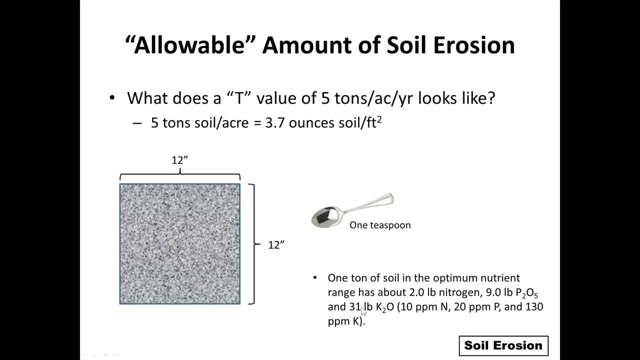 so that's right in the middle of a nutrient range. you could be losing, with each ton of soil, about 2 pounds of nitrogen, 9 pounds of P2O5, and 31 pounds of K2O. So if you add that up, multiply that by 5,. 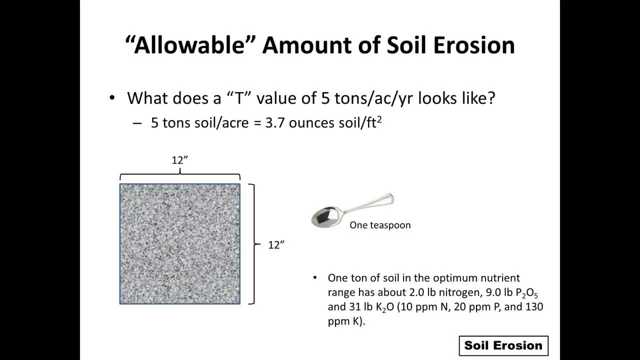 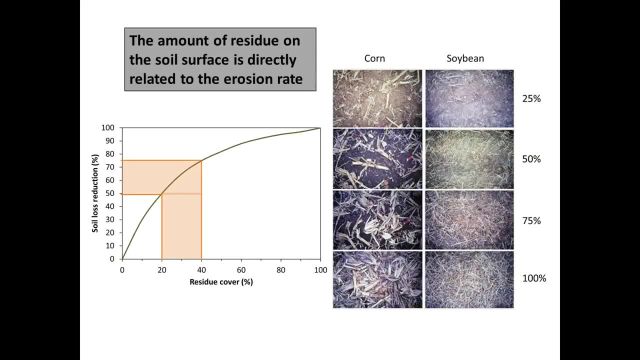 you know, and you then try to replace the fertilizer, it can have a fairly large economic impact. So when we're looking at soil erosion by water, we know that residue- crop residues- are our best defense And the amount of residue that we have on the soil surface directly relates to the amount of erosion. 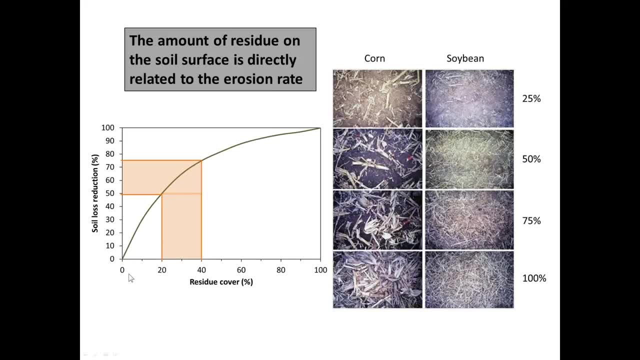 So here's an example on this graph here on the left side of the screen: Residue cover on the horizontal axis. on the vertical is the soil reduction. We know that about 30% residue cover will reduce erosion to about 50%. On the right side I have an example, or looking at examples, of corn and soybean residue. 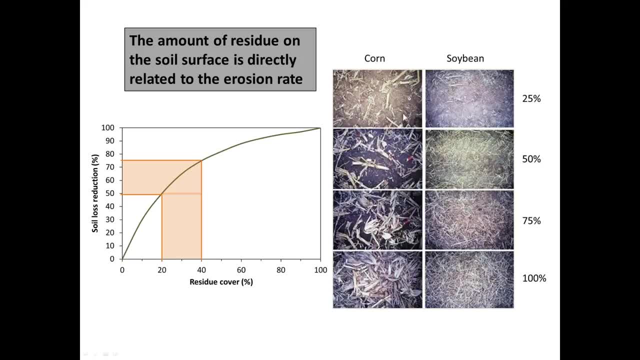 What does 30% residue look like? Here, on the top one we have 25%. That's pretty close to 30. You can see it doesn't take a lot of residue and we can make some nice steps forward towards reducing erosion. 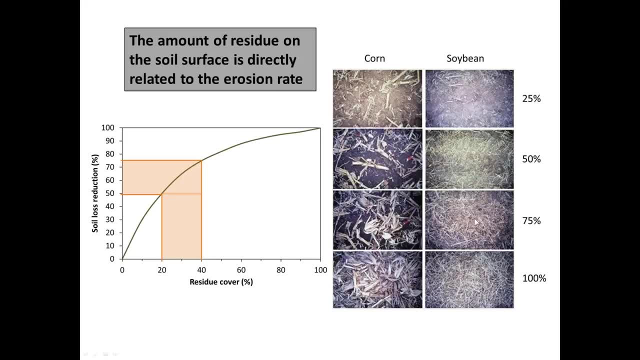 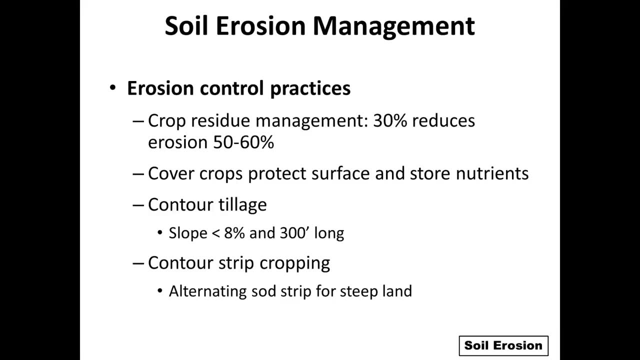 50%, even 50% residue doesn't look like a whole lot. 75% and 100% residue. So let's talk a little bit about erosion management. So what practice? what things can we do to control or manage erosion? 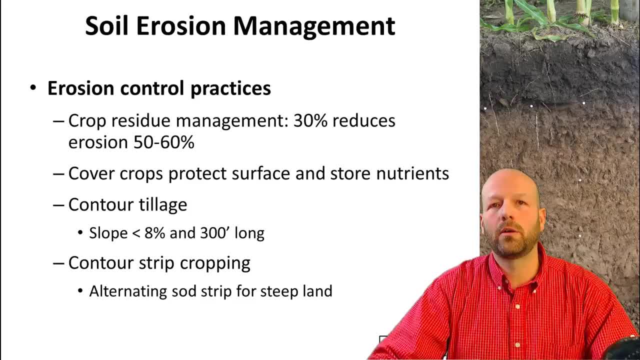 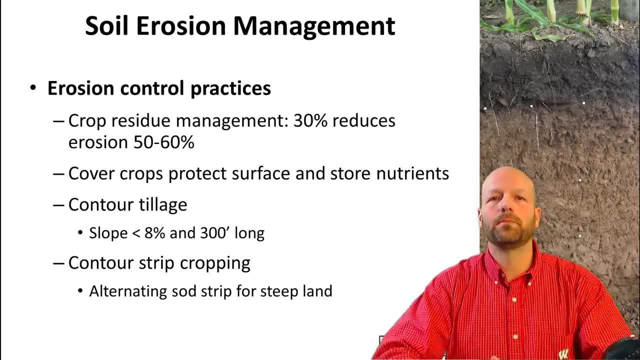 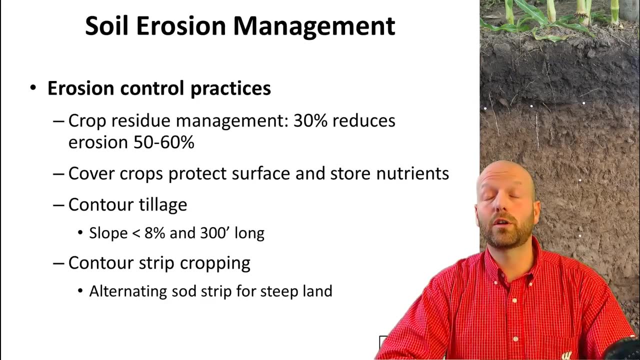 Again, like I said before, 30% residue on the soil surface can reduce erosion by 50% to 60%. Obviously, that's going to depend on different conditions. Cover crops can be a great way to protect the soil when it's the most vulnerable. 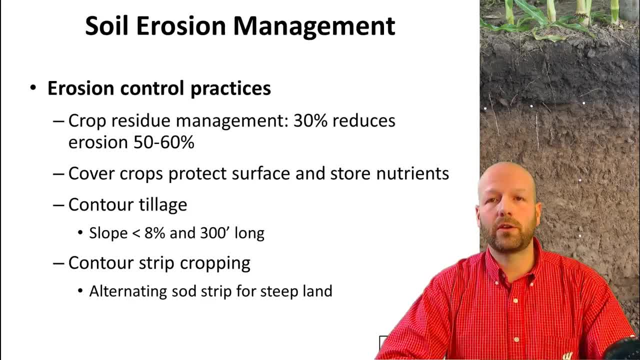 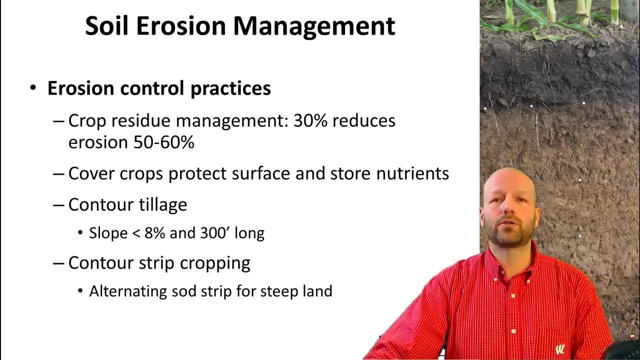 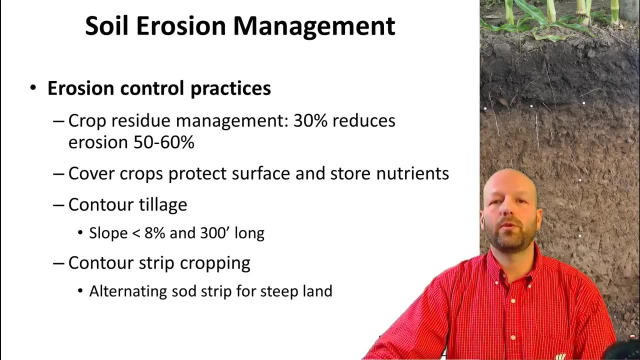 And it also helps recycle nutrients and other benefits, with biological benefits and such that we talk about, We're aware of. Another way to control erosion would be by doing tillage on the contour. This could be quite beneficial, And another way would be using contour strips for cropping. 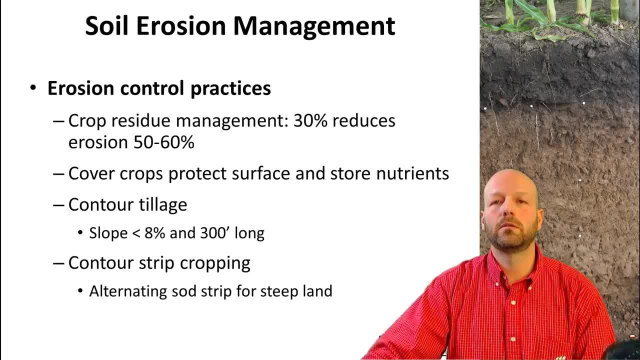 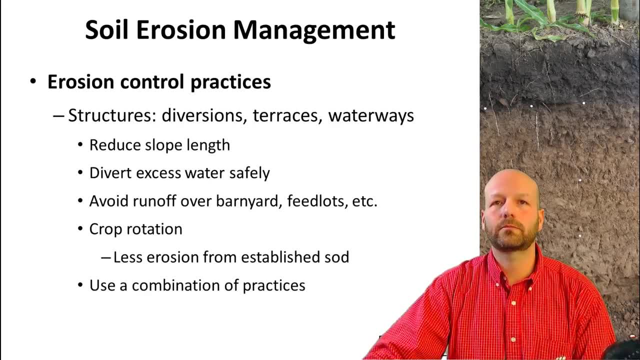 And so, basically, you alternate strips of different crops, including sods, to break that slope on the landscape. Other ways or different structures that could be used for erosion control include erosion diversions, terraces, waterways. So a lot of this if you think about it. 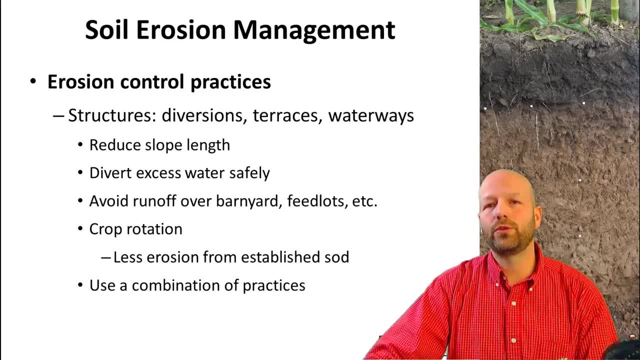 think back to that USLE equation that we talked about. What they're trying to do is modify some of those factors. In this case, it's the LS factor, the slope. So in this case, this practice is aimed to reduce the slope length. 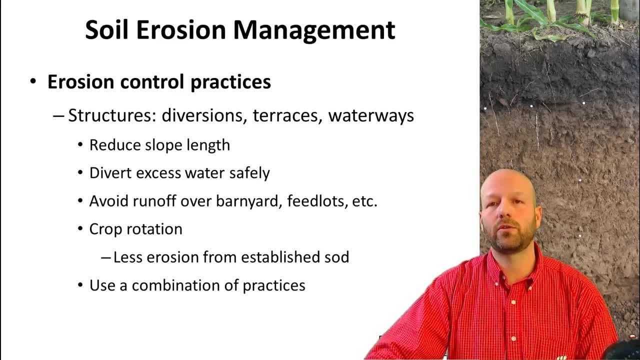 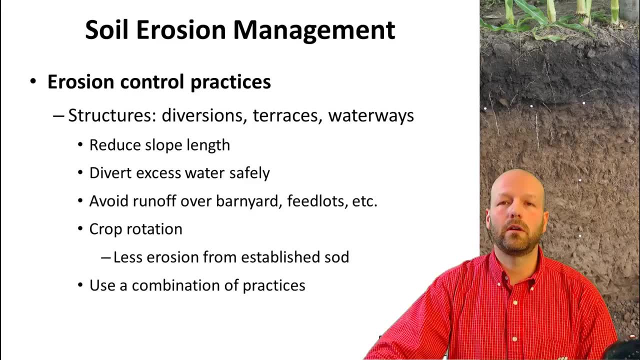 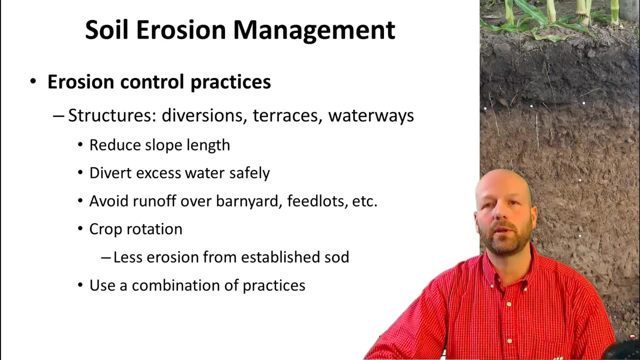 divert water safer, So they're trying to avoid any confluence of water concentrated flow. Another way of improving erosion management is to avoid runoff on feedlots or barnyards, where we know that that area is going to be compacted So it's going to have very poor infiltration. 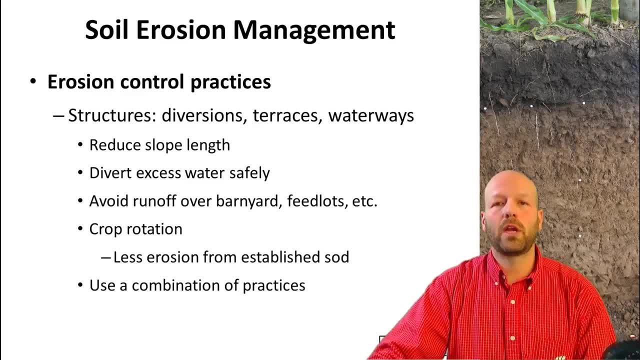 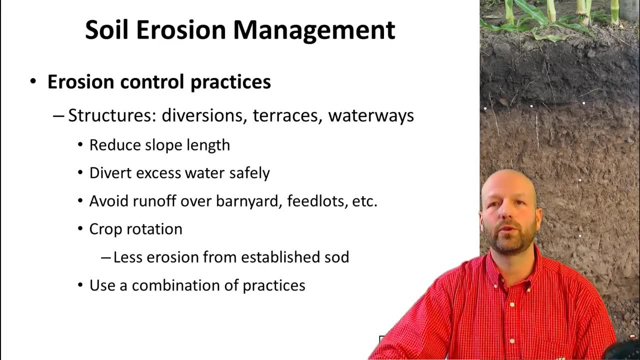 We have more water moving out of those areas. Crop rotations can be important, too to control erosion. If you include a crop that has a lot of residue or a different root structure will help hold that soil in place And, ultimately, the best way to control erosion. 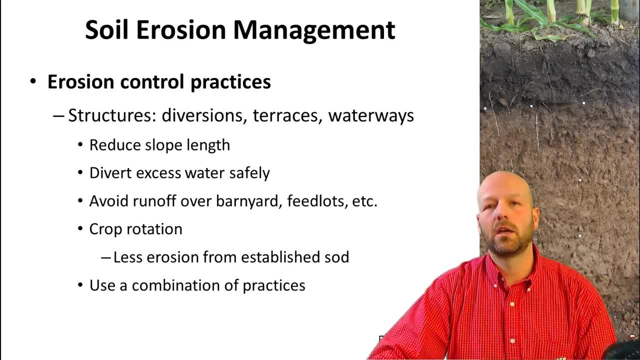 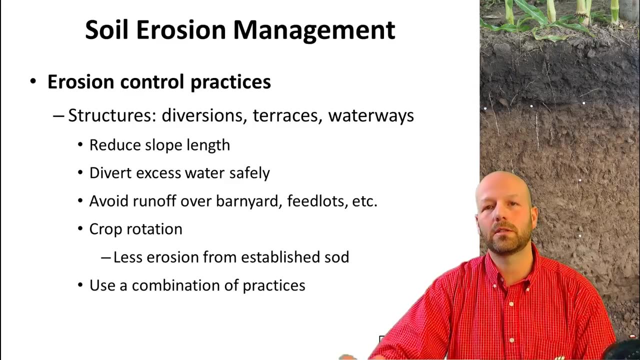 is actually using a combination of different practices. So trying to reduce the tillage, including residue management techniques, including cover crops- If you have steep slopes, contour cropping and all those type of things as a whole, as a package, can be very effective in reducing erosion. 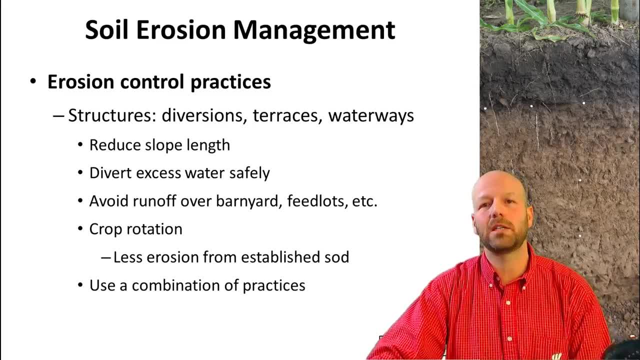 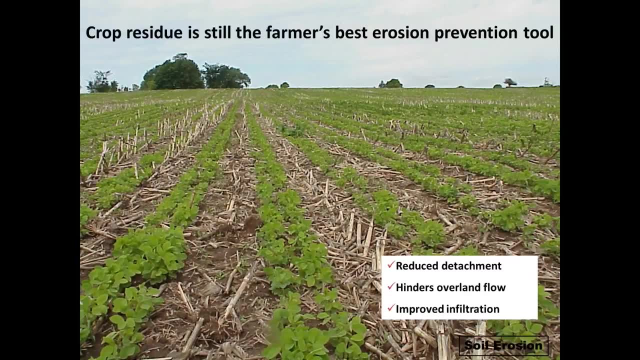 So these are not new techniques. This is basically back to the basics. We know that these are very effective and have been used for decades. Again, I have to reiterate the importance of crop residues. It is the best tool that we have for controlling erosion. 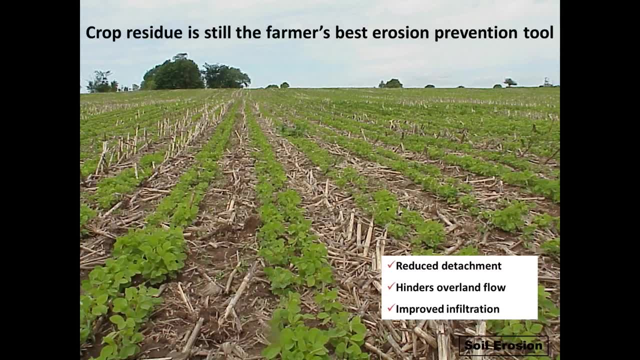 simply because it's protecting that soil surface from the impact of raindrops. So it's trying to reduce or avoid that first step of erosion, if you recall, which is the detachment of the soil particles. So it's very, very important to protect that soil surface. 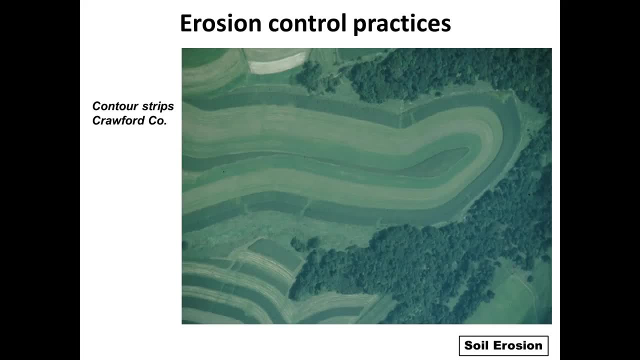 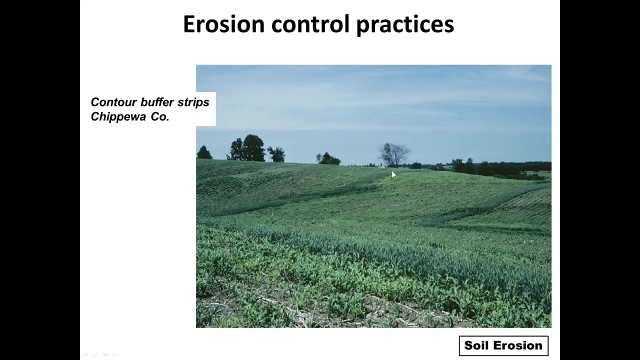 Here are some examples of different erosion control practices, Just for your review. here are some contour strips. As you can see, they basically follow the lay of the land or the landscape. These are buffer strips, A little bit difficult to see, but you see there every so often. 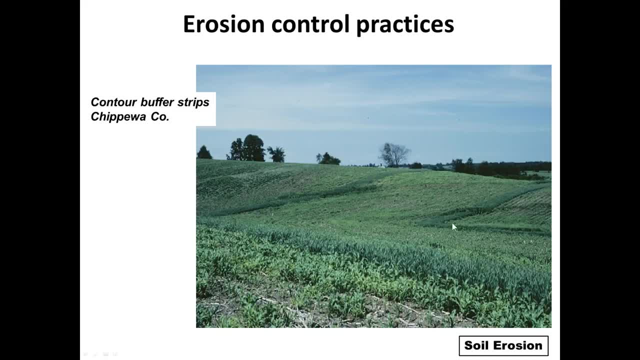 There's these strips with a grass buffer area that it's helping break down that slope and reduce the slope length. So if you have any runoff it would slow that water as it goes down the slope. Here are terraces. Essentially, terraces are again breaking that slope. 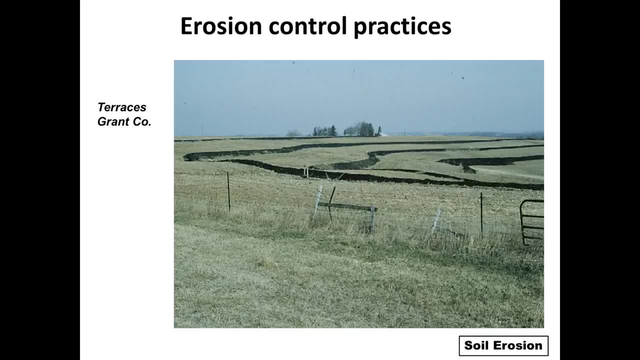 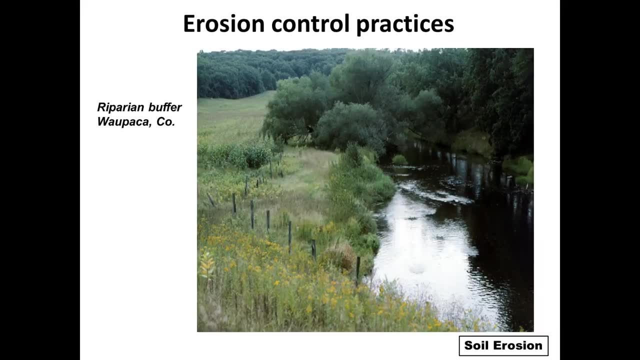 but also changing the slope of that field. So it's kind of a double effect that we see here, And repairing buffers are kind of, in my view, kind of a last-ditch effort, in that they're going to be right very important. 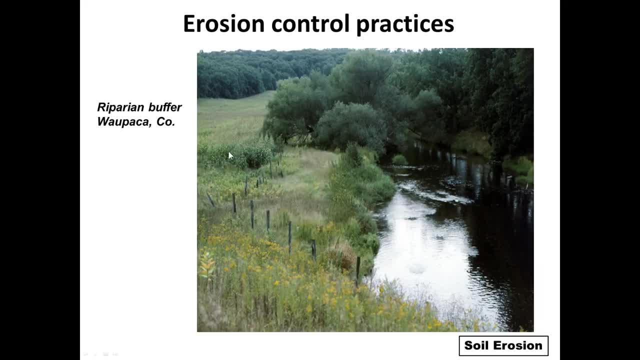 but they're going to be right next to a creek. So if you have any water moving from the field that is going to end up in that creek and it's carrying any sediments, these buffer strips are very effective at reducing the speed of that water. 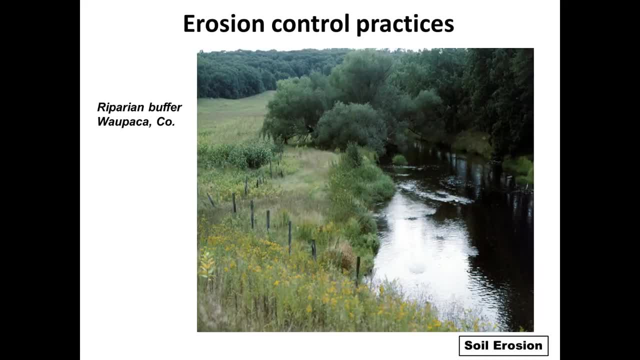 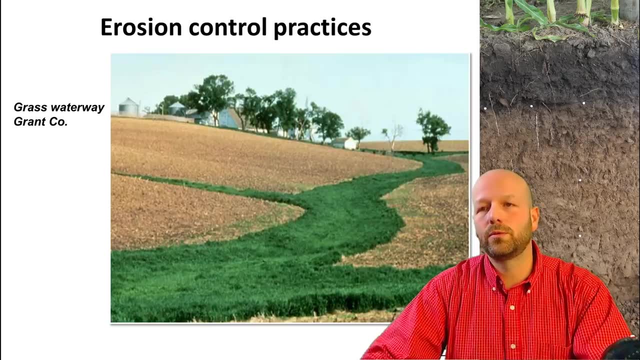 and then allowing those particles to settle out out of that water and not reaching the stream. Another important one that I have to really stress is the use of grass waterways. They're very effective at removing water- excess water- from the field in areas where we get concentrated flow. 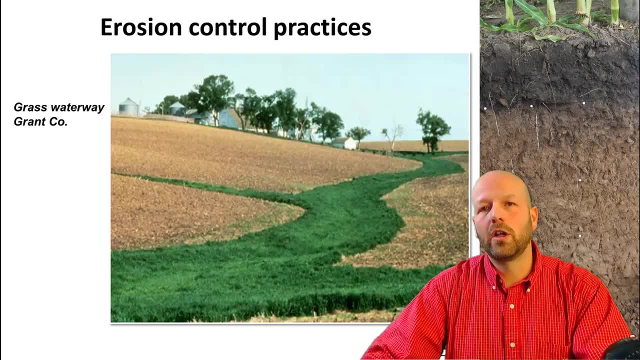 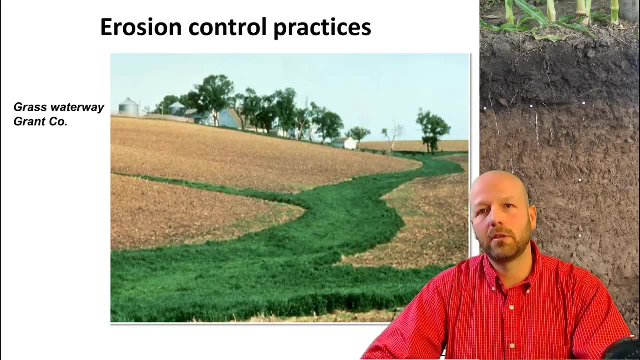 and they also help to avoid gullies and rills in those areas. So they're very, very effective at controlling erosion in specific areas. I realize they can be sometimes a little difficult to manage and can be a problem, but they are very important.